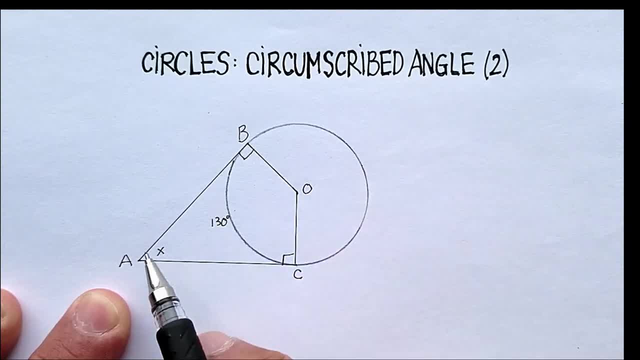 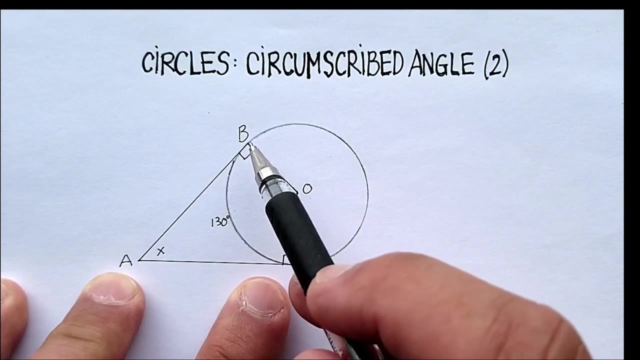 Okay, so remember that's very important. Circumscribed angle vertex outside the circle. In this case it would be point A. Now it forms two tangent lines with the circle itself, And remember that tangent lines form 90-degree angles with the circle. 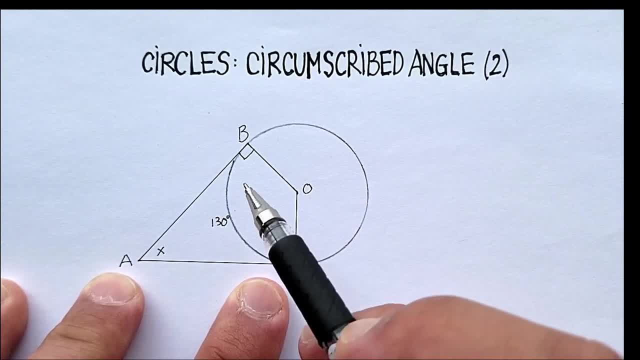 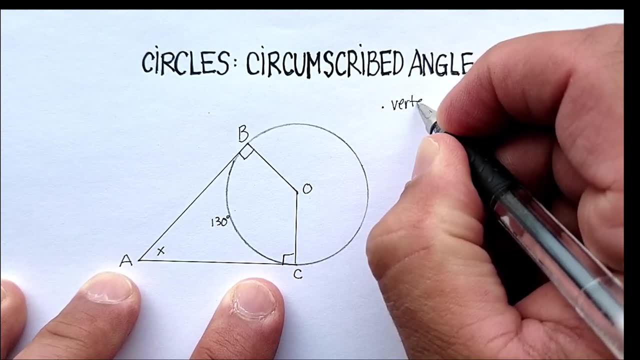 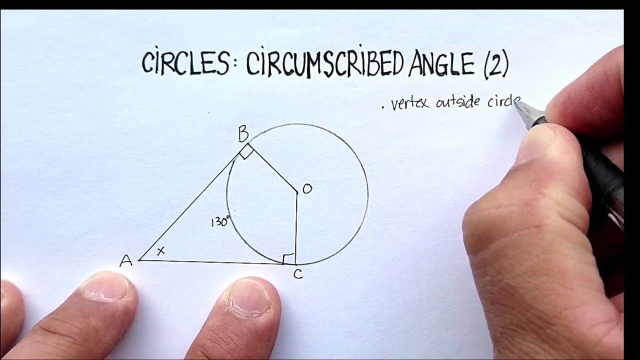 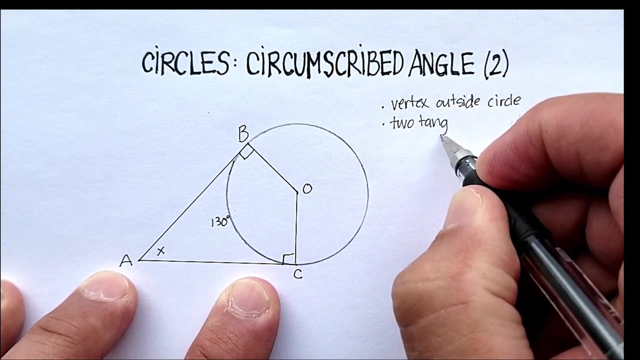 So to the center of the circle. this angle here would be 90 degrees. Let me just write all that down again. So first property: vertex outside circle: Okay, Very important. Second property: two tangent lines. There we go. 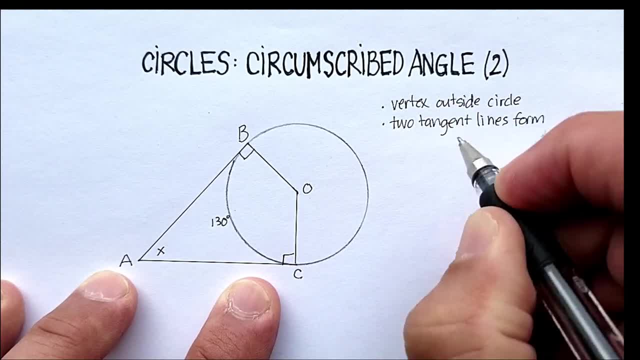 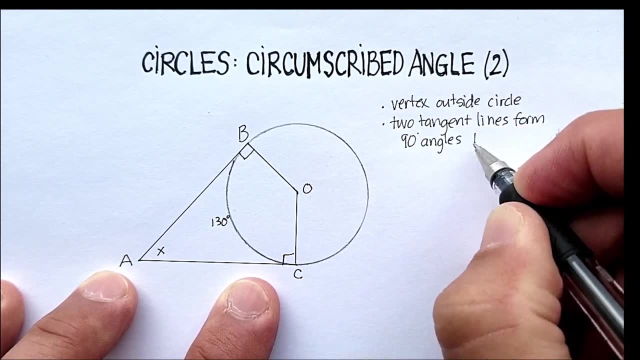 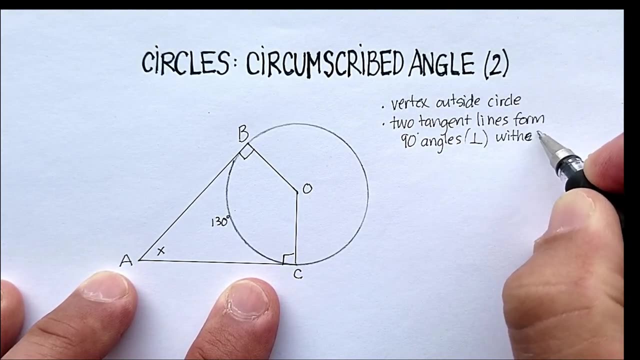 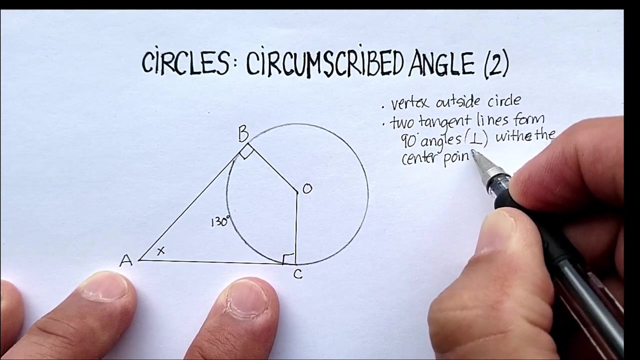 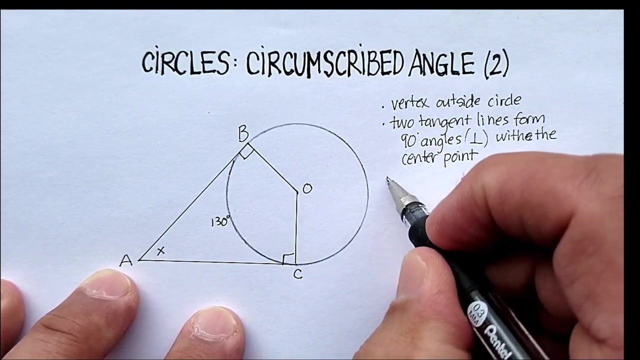 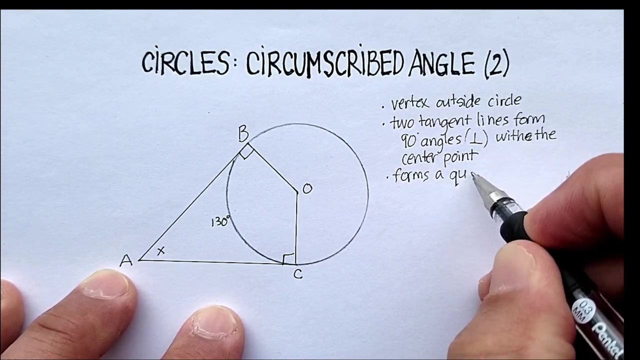 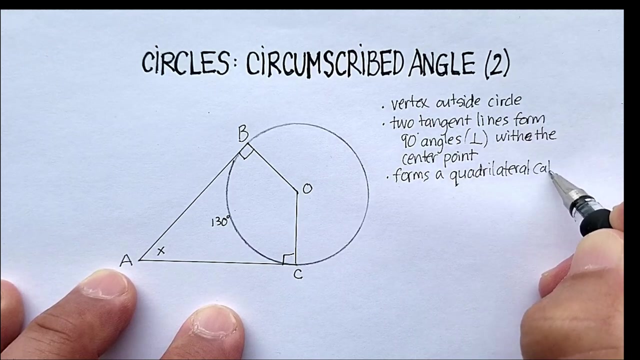 Which form 90-degree angles or perpendicular angles- Remember, that's a symbol for perpendicular- with the center point Whoops. In this particular case, we will form a kite right, A four-sided figure, So it forms a quadrilateral called- that's a Q- quadrilateral called a kite. 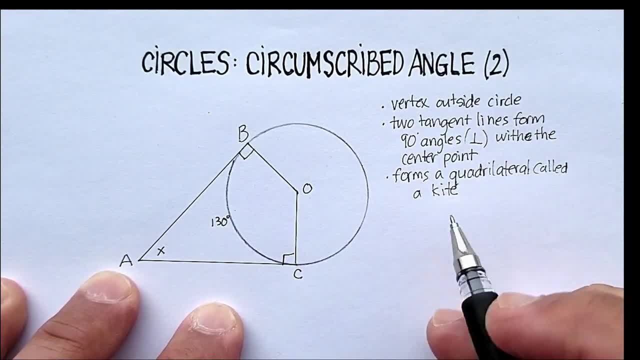 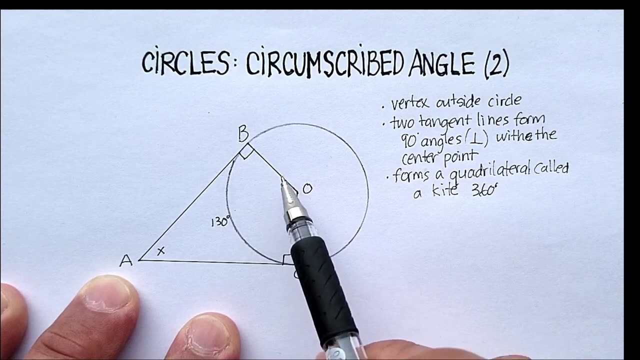 Now you know that any four-sided figure has 360 degrees internally, or internal angles, right? So one thing that you could do to figure out the angle or the measure of a circumscribed angle is to add up all three of the other angles and subtract from 360, right? 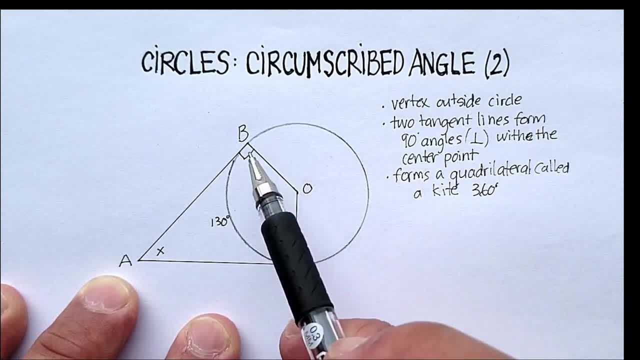 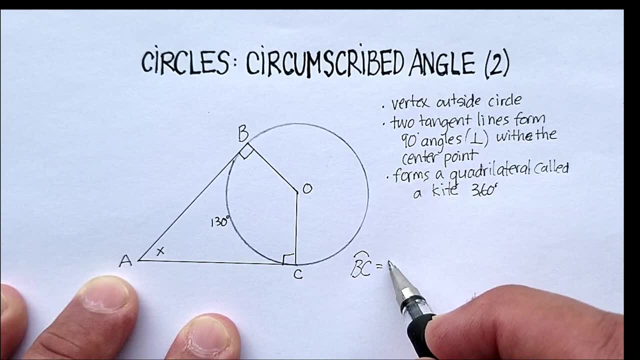 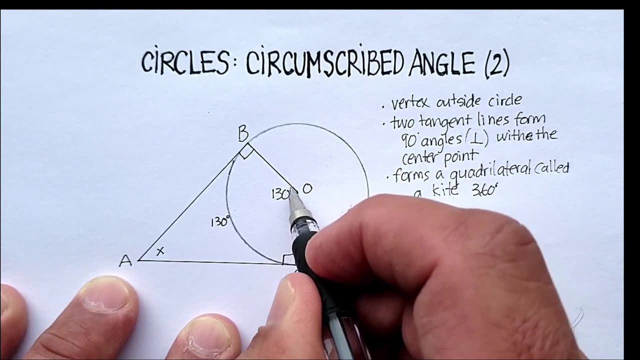 And you need to know the third angle. In this particular case, I know that arc A or BC rather equals 130 degrees, which means that my central angle- different word, central angle- is 130 degrees. Remember, central angle starts in the middle. 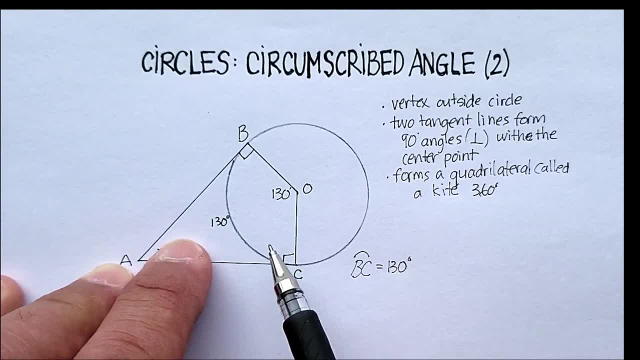 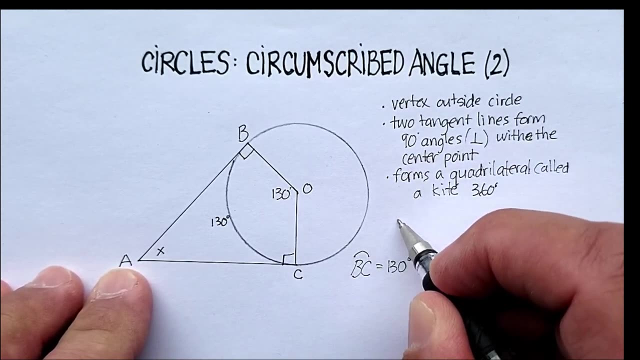 The vertex starts in the middle of the circle. So I could just add up 90 plus 90 plus 130, and I could find my circumscribed angle. The other way to do this is the second method. So I know that opposite angles- and this is the important part of this particular video.